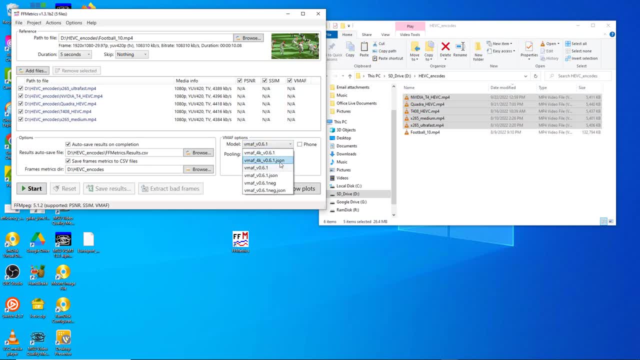 you choose the model. You can choose either the JSON or the PICL model, It doesn't really matter. And then you can pool using the harmonic mean or the mean. I prefer the harmonic mean and this, obviously is how you would select the phone model Once you get all that set. 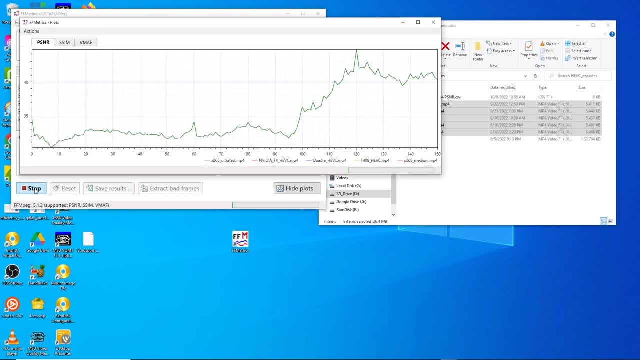 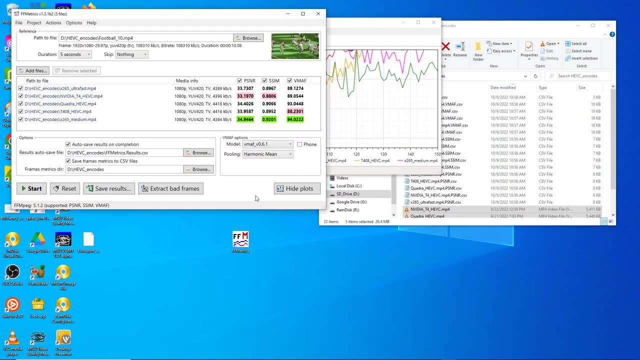 up, you click Start and the program runs. I'll come back once all the data is filled in. So we are all done And what you see here is the program And what you see here and just by way of background, I'm analyzing the quality of 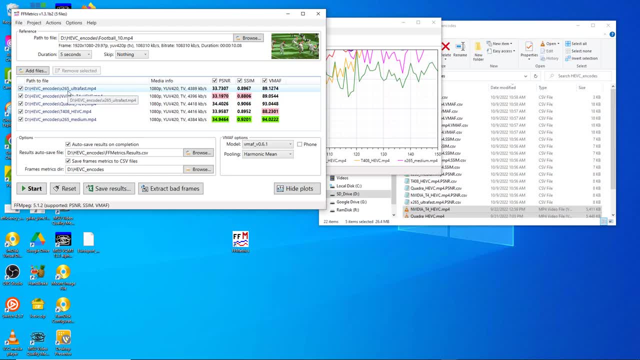 five files encoded using the HEVC codec. This is X.265 using the ultra-fast preset. This is NVIDIA T4.. This is Quadra and T408.. Those are NetInt products and this is X.265 Medium. And you see the scores here. These are average scores and I'll show you some more detail. 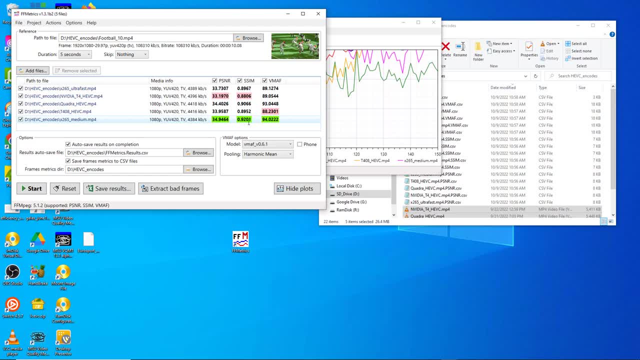 in a moment And the best score in the group- in this case it was Medium- is in green and the worst score in the group is in green And the worst score in the group is in green And the worst score in the group is going to be in pink And, if you want to hover over, 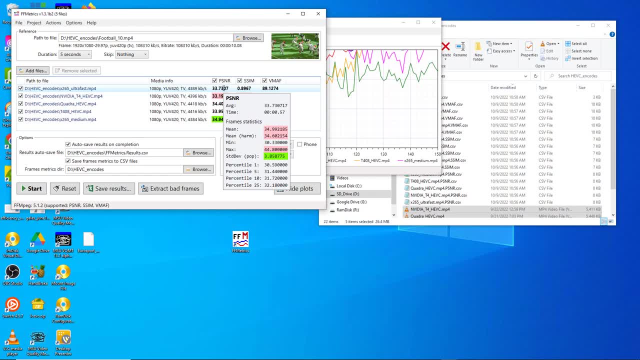 the score itself, you'll see more information about the score, including the mean score, the harmonic mean score, minimum frame, maximum frame and standard deviation, as well as the percentile data. Most of this information is going to be available in either the frame. 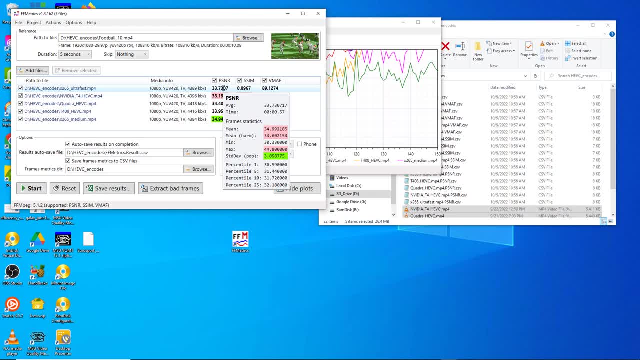 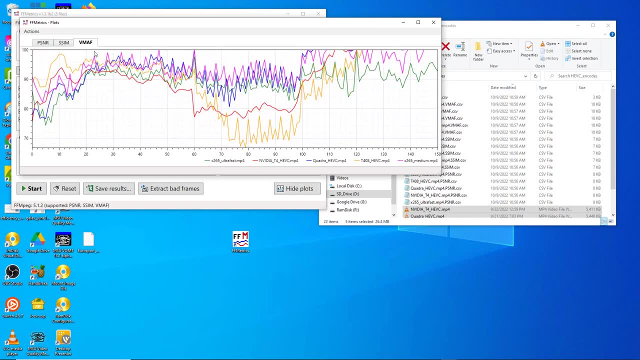 file or the results file that we'll look at in a moment, And this is the plot and there's a separate plot for PSNR, SSIM and VMAPH And you can zoom into the plot using your mouse wheel and then click your right mouse button to. 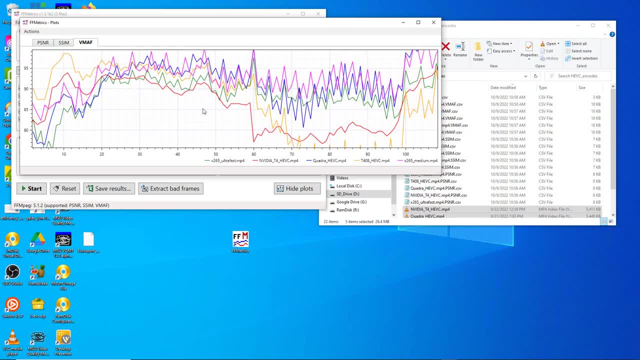 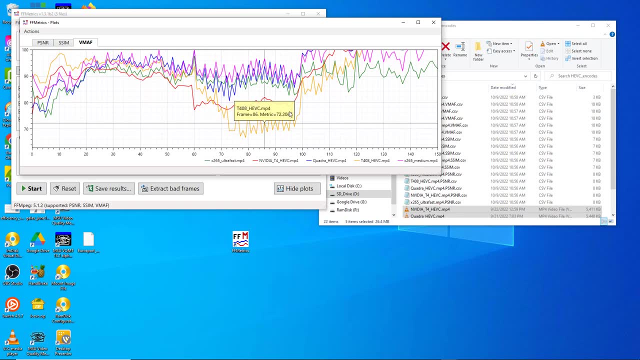 kind of zoom around At any point in the video. you can click down here and see that this frame came from the T408.. And let's go to This frame came from the NVIDIA and you can see the frame number and the metric. So let's. 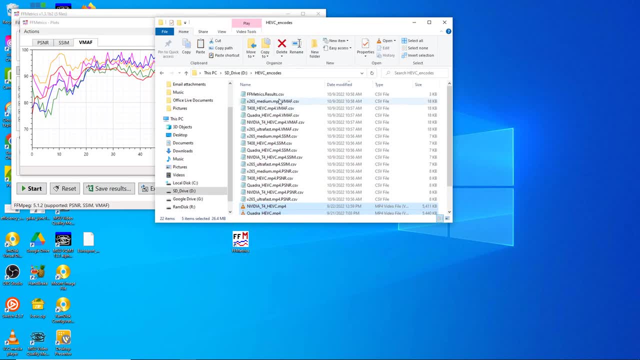 go to the results files themselves. So we see a bunch of results here. This is the general results file that's going to have all of the summary data in it And these are the individual results files for the metrics and the file that it analyzed. So this is X.265.